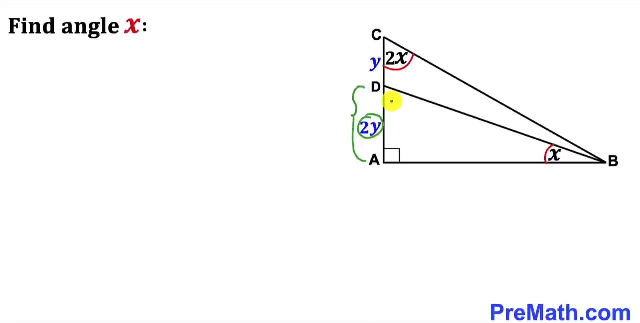 AD is 2 times Y units, and now we are going to calculate this angle X. Please don't forget to give a thumbs up and subscribe. Let me make it very clear that this figure may not be 100% true to the scale. Let's go ahead and get started with the solution, and here's our very first step. 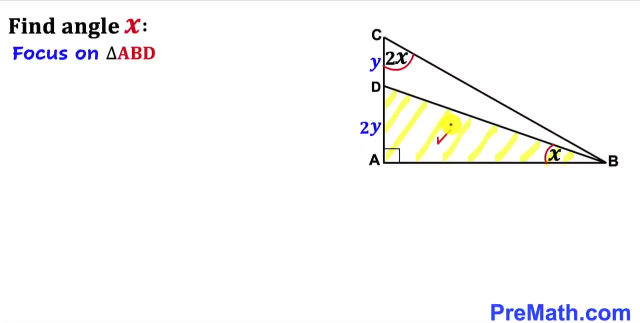 Let's focus on this right triangle, ABD. and now we know that this is our 90 degree angle and this is our angle X and we want to figure it out. This angle, I'm going to call this angle alpha. and now let's recall triangle sum theorem: The sum of 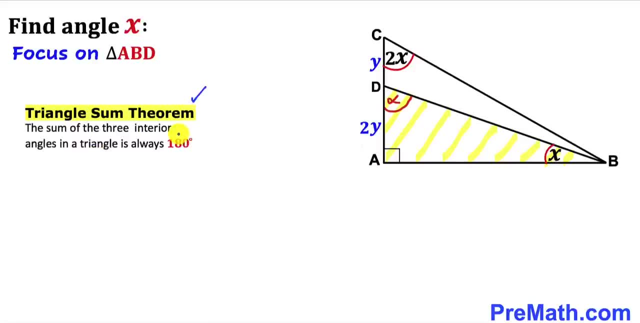 the three interior angles in a triangle is always 180 degrees. so therefore the sum of all these three angles must be equal to 180 degrees. So let me go ahead and write down: 90 degrees plus angle alpha, plus X is equal to 180.. 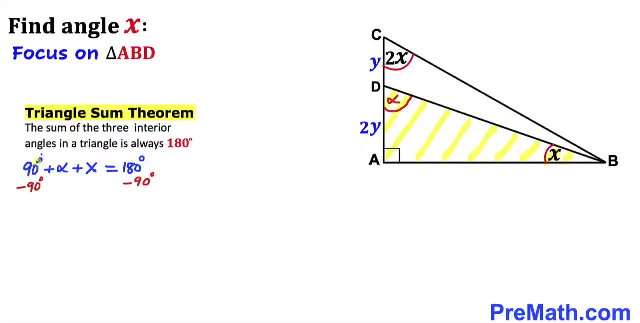 Subtract 90 degrees from both sides, This is gone. So therefore, alpha plus X turns out to be 90 degrees on the right hand side. Let me go ahead and move this X on the right hand side, So our angle alpha turns out to be 90 degrees minus X. 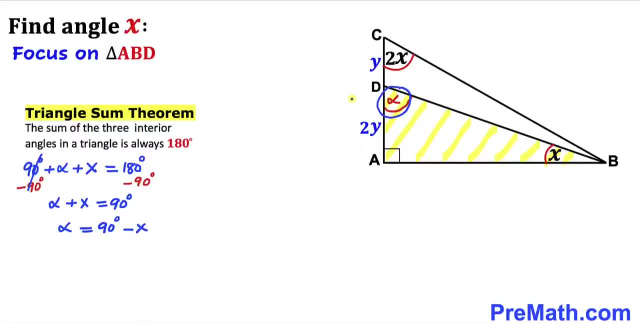 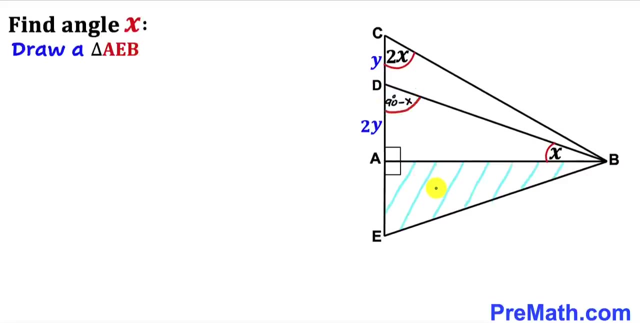 So, therefore, our this angle alpha turns out to be 90 degrees minus X. So, therefore, our this angle ADB turns out to be 90 degrees minus X. And here, in this next step, we have drawn this right triangle AEB by extending: 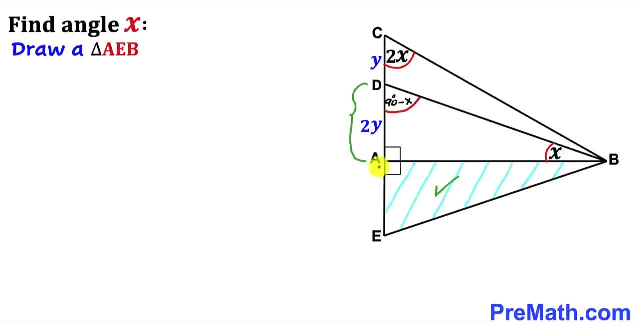 this line segment AD by 2Y over here and now let's focus on these two right triangles, ABD and this right triangle EBA. we can see that this angle is 90 degrees. this angle is 90 degrees as well. moreover, this side length AD is 2 times y and this side length EA is. 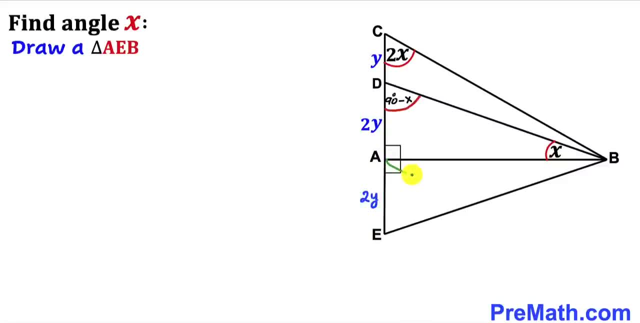 2 times y as well. and finally, this side length AB is in common between these two triangles. so therefore, we conclude that these are two triangles: ABD and this other triangle, AEB, are congruent triangles according to side angle, side congruency theorem, and since these 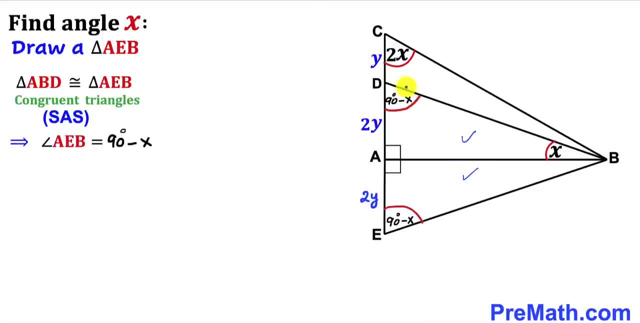 two triangles are congruent, so therefore, this angle has got to be equal to this angle. so therefore, our this angle, AEB, turns out to be 90 degrees minus x and finally, if this angle is x, this angle has got to be x as well. as you can see over here. 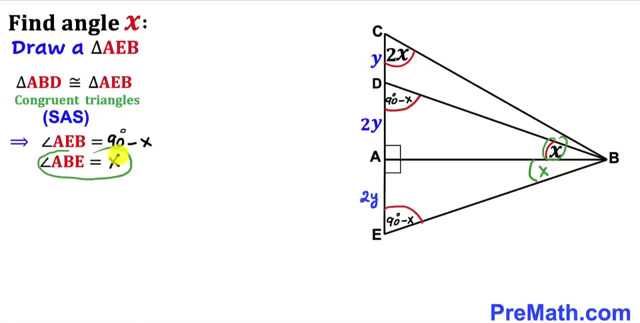 our angle a, b, e is x. and now, in this next step, let's focus on this bigger triangle e, b, c, whose angles are 90 degrees minus x, 2, x, and let me go ahead and label this whole angle as our angle theta. and now let's recall this triangle sum theorem once again: the sum of 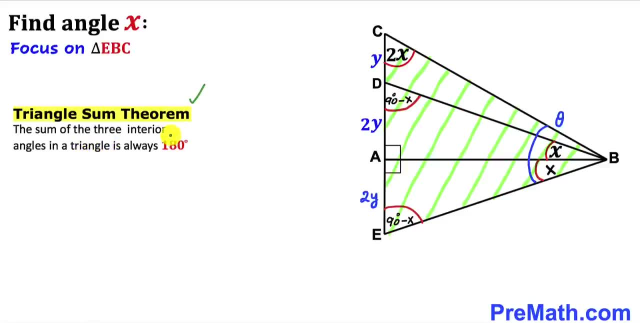 three interior angles in a triangle is 180 degrees, so therefore let me go ahead and add all these three angles: 2x plus this angle plus angle theta. so let me go ahead and write down angle 2x plus angle 90 degrees minus x plus this angle theta. 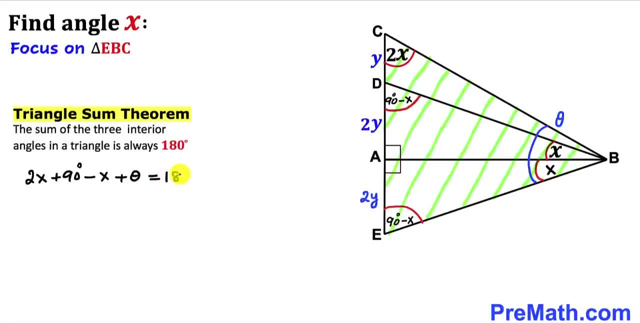 so, so, so. so they must be equal to 180 degrees. now let's go ahead and subtract 90 degrees from both sides. this is gone. and here, if we combine these two angles, or 2x minus x, that is going to give us angle x plus theta on the left hand side equals 2 on the right hand side is going to give us. 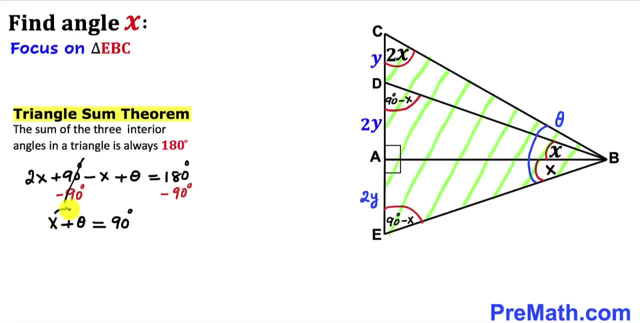 90 degrees. now let's go ahead and move this x on the right hand side. so, therefore, our angle theta turns out to be 90 degrees minus x. so, therefore, our this angle theta turns out to be 90 degrees minus x. and now let's go ahead and make an observation in this big triangle: ebc. 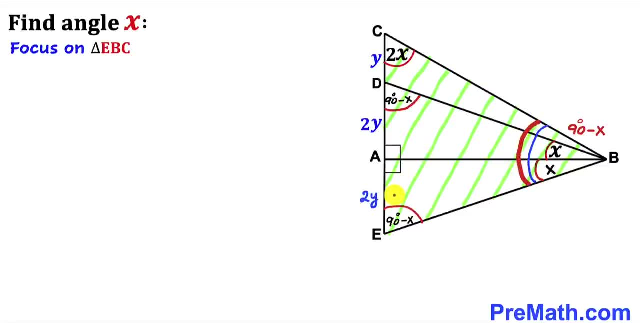 we can see that this whole angle is equal to this angle. both of them are 90 degrees minus x. so therefore we conclude that this triangle, ebc, is an isosceles triangle. in other words, this side length is equal to this side length. in other words, this ec is going to be equal to bc. and now we can see. 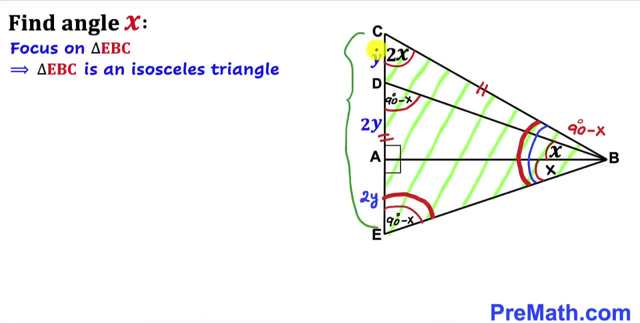 that this whole side length ec is going to be y plus 2y plus 2y. that is going to give us 5 y, and if this side length is 5y, then this side length bc has got to be 5y as well. so therefore, 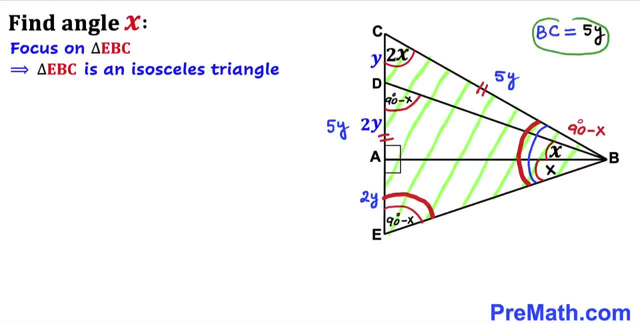 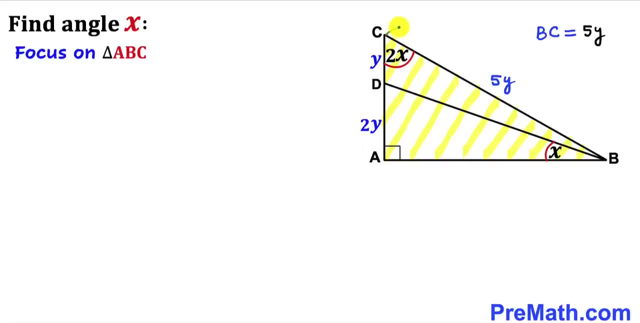 our this side length bc turns out to be 5y. and here's our next step. let's focus on this triangle abc. now we know it's this side length bc is 5 y and this side length ac is going to be y. all right, y plus 2 y. that is going to give us 3 y. and now we want to figure out this side length a, b. so we 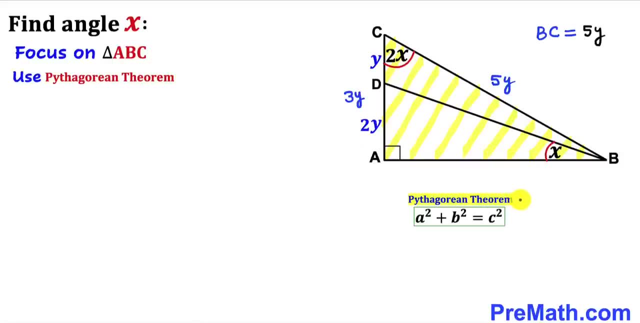 are going to apply the Pythagorean theorem. and here's our Pythagorean theorem: a square plus b square, equal to c square. let me go ahead and call our longest leg as our side c. I'm going to call this side a and this side b, so let's go ahead and fill in the blanks in this Pythagorean formula. 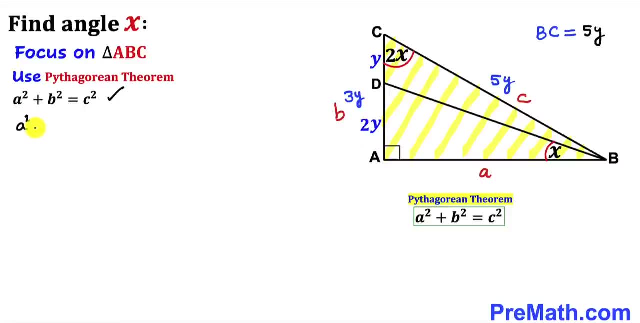 a. we don't know a. I'm going to write down a square. b in our case is 3 y whole square equal to c. in our case is 5 y whole square, so this could be written as a square plus 9 y square, equal to 25 y square. let's go ahead and subtract 9 y square from both sides. this is gone. 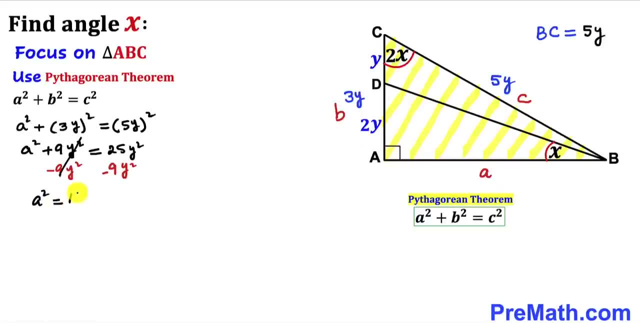 so a square turns out to be 16 y square. let's go ahead and undo this square by taking the square root on both sides, so a turns out to be equal to 4 y. so therefore, our this side length, a turns out to be 4 y. and now let me show. 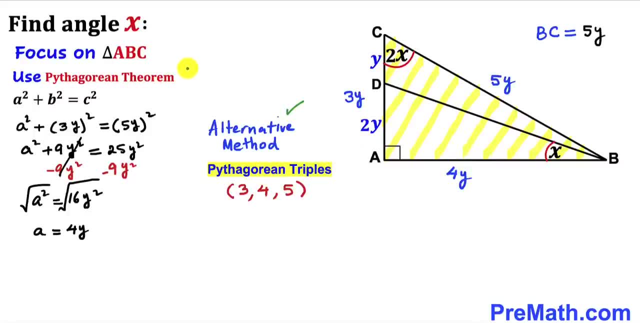 you an alternative method: instead of using this Pythagorean theorem, we could have used this Pythagorean triplets: 3, 4 and 5. in other words, in this right triangle, a, b, c, if this side length is 3 y, this is 5 y. this has got to be 4 times y. and here's our final step. 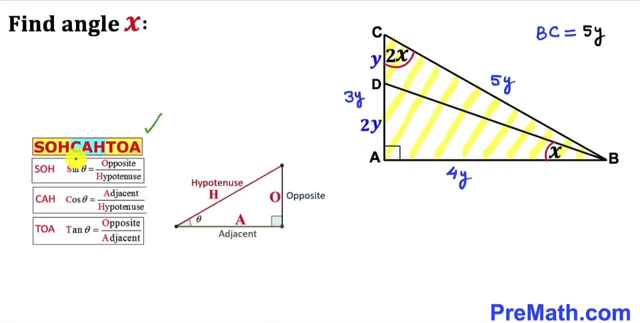 let's recall this so-ca-twa and let's go over this sine of theta- equal to opposite over hypotenuse. so therefore, if in this triangle a, b, c, if I call this whole angle theta, then this side is going to be opposite and this is longest leg. so let's go ahead and fill in the blanks in this Pythagorean. 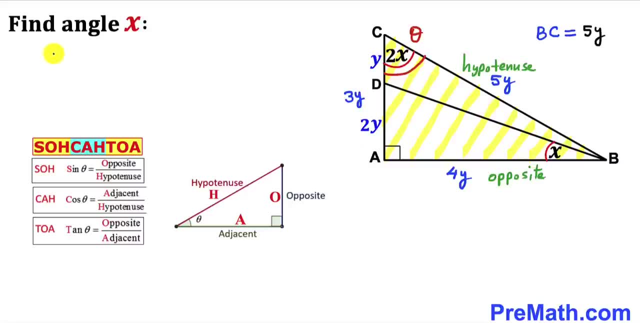 triplet. so this is going to be our hypotenuse. so therefore, sine of our angle, theta is going to be opposite. in our case is 4 y and hypotenuse is 5 y. let me go right down: 4 y divided by 5 y, and here: 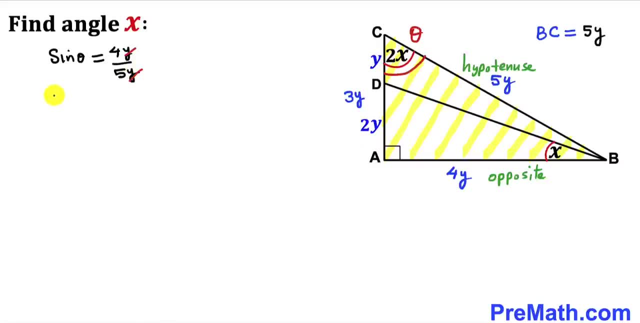 we can see this: y and y is gone. so therefore sine of theta turns out to be equal to 0.8. on the right hand side, let's go ahead and write it down as theta equal to sine inverse of 0.8. so therefore our angle theta turns out to be approximately equal to 53.13 degrees. but we know. 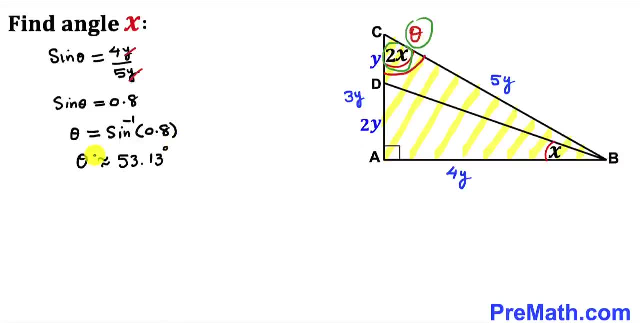 our angle theta is equal to 2x, so I'm going to replace this theta by 2x, so therefore I can write: 2x is approximately equal to 53.13 degrees. let's go ahead and divide both side by 2, so therefore our angle x is going to be approximately equal to 26.57 degrees. so 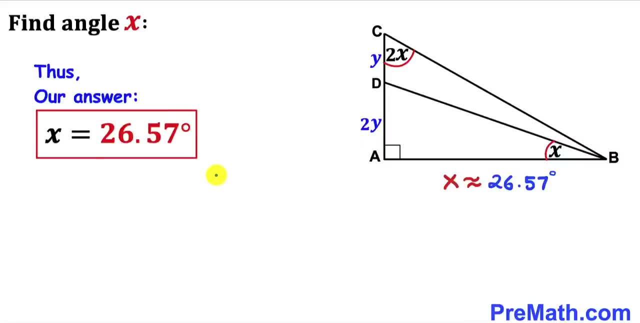 therefore, sine of theta is going to be approximately equal to 2x. so, therefore, sine of theta is going to be: